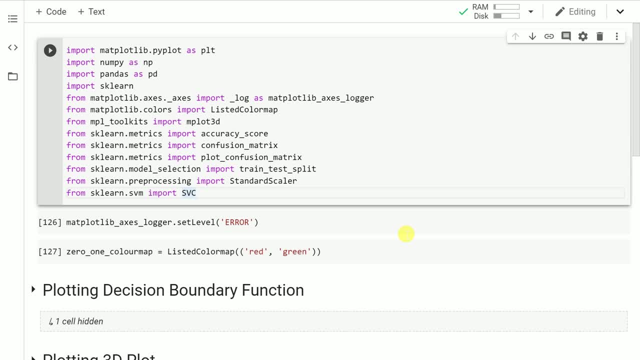 which kind of takes the data in one extra dimension and kind of creates a linearly separable data for us. What we mean to say by that is what we'll discover in this video. So first let's start by importing all the necessary modules, Apart from the necessary. 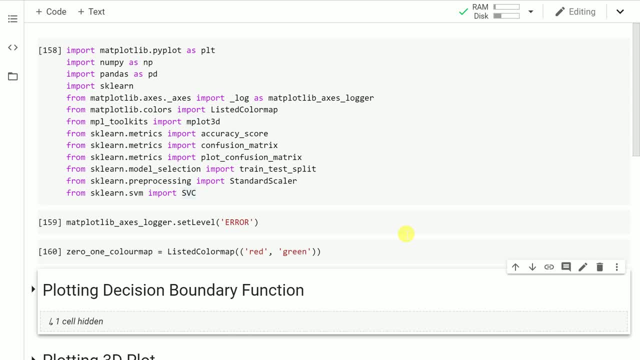 modules. I've also created something called as a listed color map to differentiate between the classes 1 and 0. In the context of this example, the samples with the target value being equal to 0 will be displayed as a red color dot. On the other hand, the samples 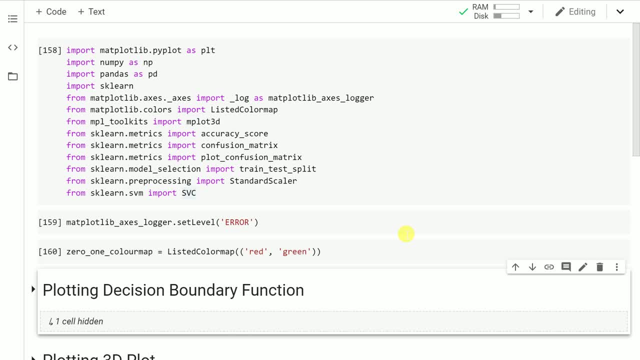 with the value 1 would be displayed as green color, And I've saved this color map into a variable called as 0 underscore, 1 underscore- color map. Where do we utilize? this is what we'll discover in the coming functions, as well as the code that I kind of walk you through. 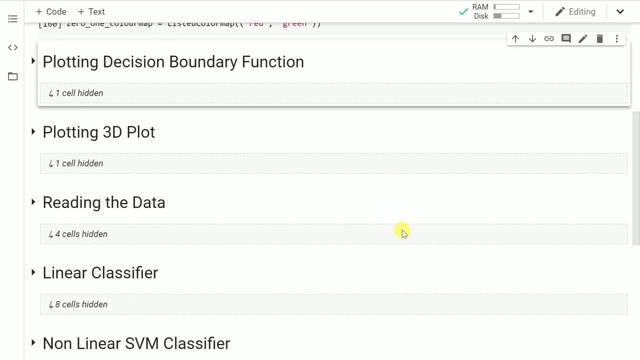 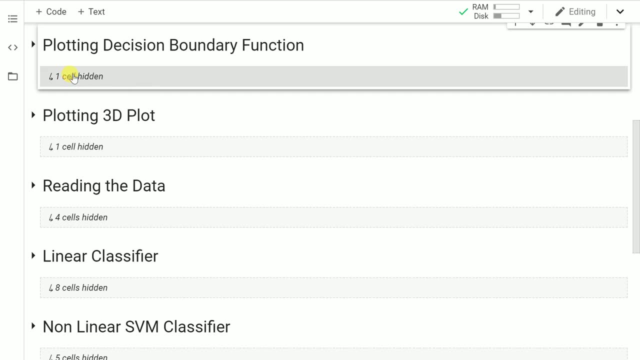 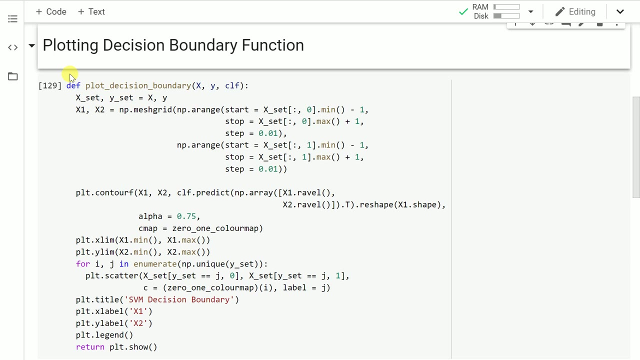 So let's proceed forward. First things first. I've created a simple function, So let's start with a simple function called as plot underscore- decision underscore boundary, which takes in the x values, the y values and the classifier and helps me plot a decision boundary for. 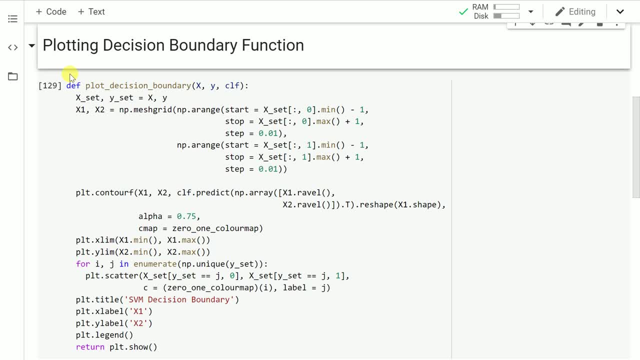 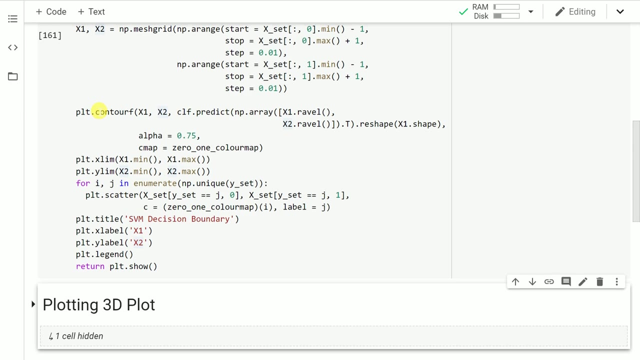 that particular classifier that is there. This is a standard way of plotting a decision boundary, So I wouldn't go in depth of explaining the function. This is kind of readily available online as well, So I run the cell to import this function into memory as well. So I've 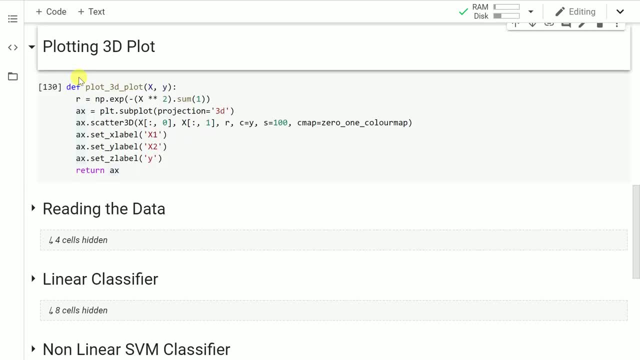 done that. The next thing that I've also done is I've also created a function called as plot, underscore 3d, underscore plot, which basically takes a two dimensional array with its target variable zero and one, And, using some transformations, helps you visualize a. 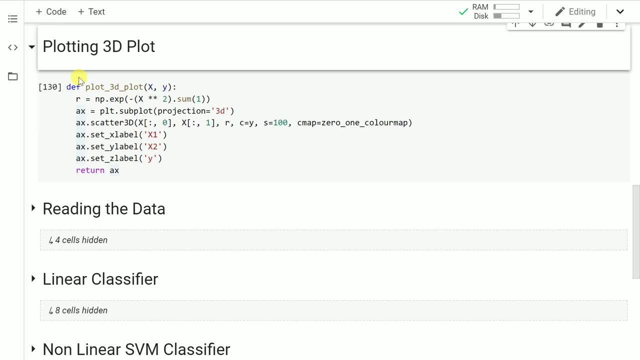 2d data by pushing some amount of data into three dimensional space. We'll uncover the magic of this function once we kind of reach at that position. But for now what I'll do is I'll import the cell into memory so that we can better utilize this function going. 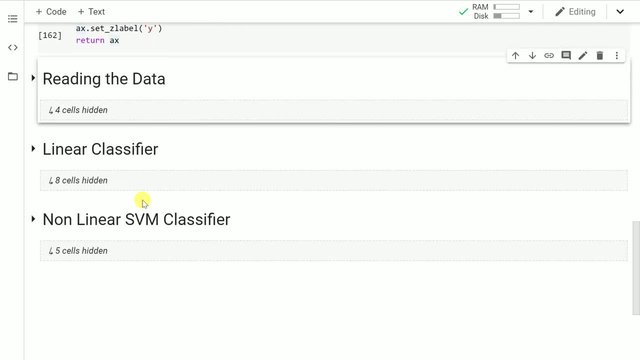 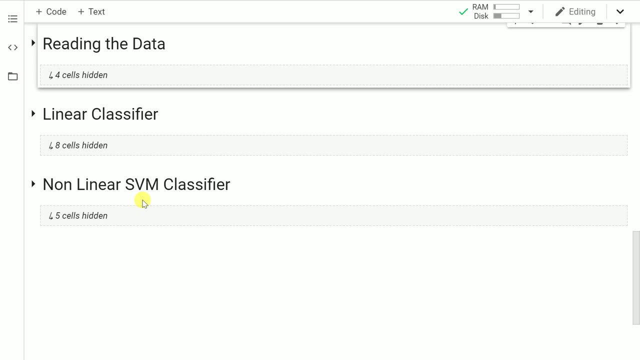 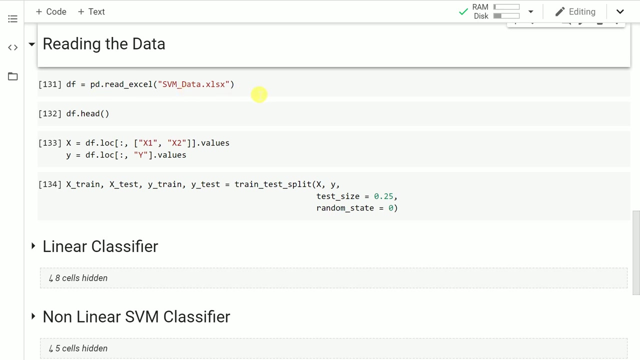 forward. Once we've imported the necessary functions in memory, we now go into the standard practice of reading the data that we have. Let's go forward with the standard practice of reading the data set. So I have a simple file called as SVM underscore data dot XLX. 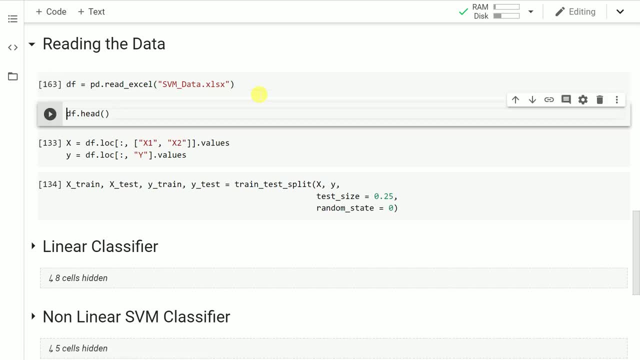 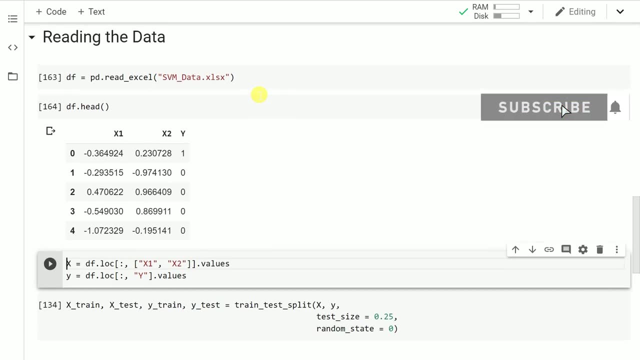 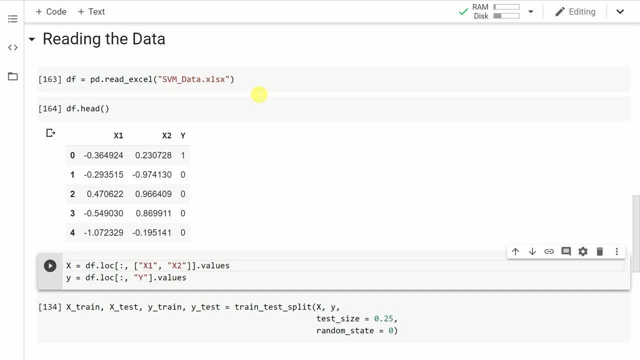 which is a simple Excel file which I load into my data frame DF. Let's visualize the first five rows of my data frame. So, as you can clearly see, my data frame has three columns: X1, X2 and Y. X1 and X2 are my feature columns, and Y is 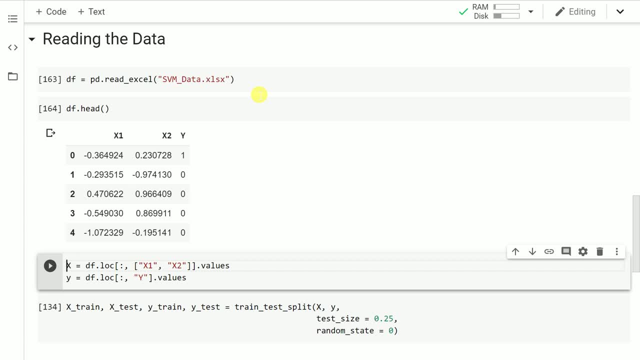 my target variable having values just zero and one. So it's a binary classification problem that I have. The standard practice going forward in a classification algorithm is to separate out X and Y. That is your features and target variable, which is what I've achieved here. So I've 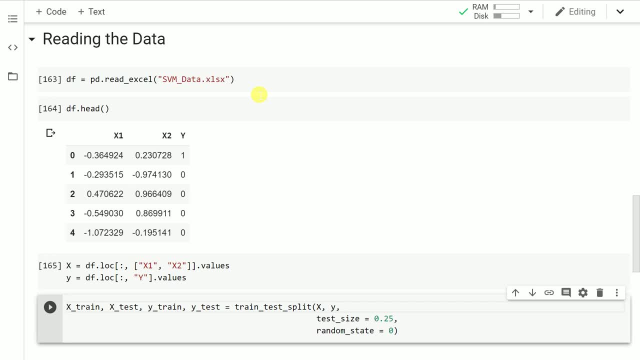 achieved in this cell. So I run the cell of splitting the data into X and Y, that is, features and target variables. Once I've splitted the data into X and Y, the next step boils down to splitting the data into training and testing, which is what I've achieved using 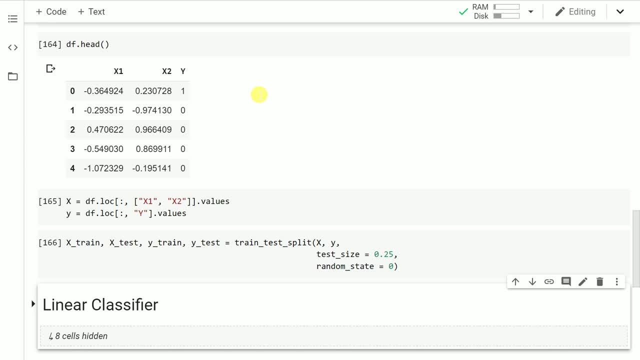 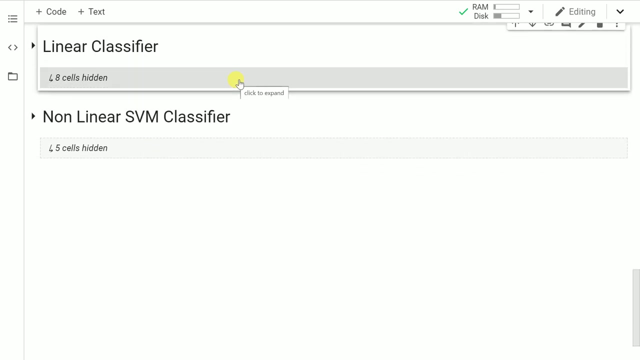 this cell. So when I run the cell I'll have, out of all the training samples that I have, 75% of the data would be used for training and 25% of my data would be used for testing purposes. Now that my data is splitted into training and testing, let's go on to the whole exercise. 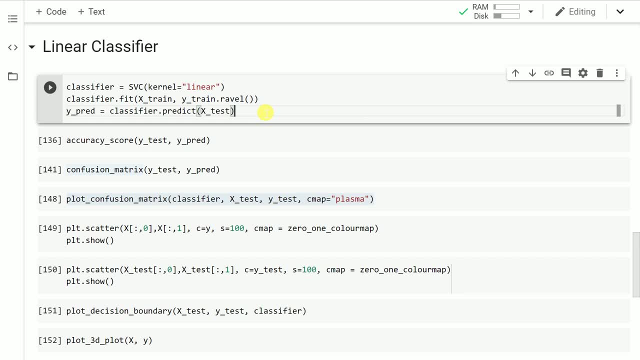 of model building. So I create an instance of the SVM classifier and also specify the kernel as linear and save it into a variable called as classifier. Now that I've defined the variable classifier, the next thing that I do is I fit the data, that is, X and Y, that 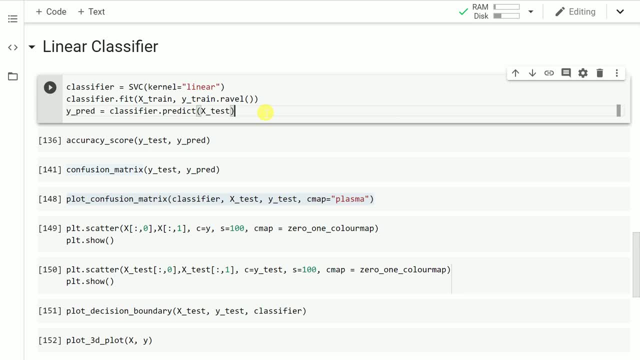 is my training data into the classifier. And once the data is fitted into the classifier, I make the predictions using the predict function of the classifier and save the predictions on the test data set- that is, X test- into a variable called as Y underscore pred. So let's run. 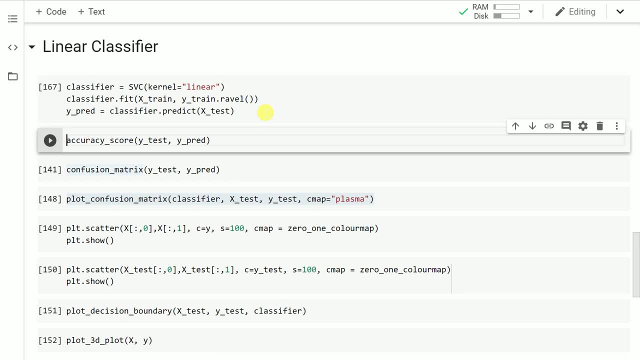 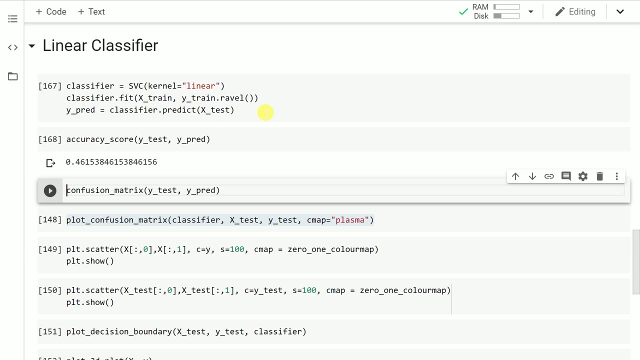 the cell. Now, as a standard practice to validate how good your classifier is performing, you have something called as the accuracy score, So let's validate how good our accuracy is After running the cell. I understand that my classifier accuracy is just 46%, which isn't great. 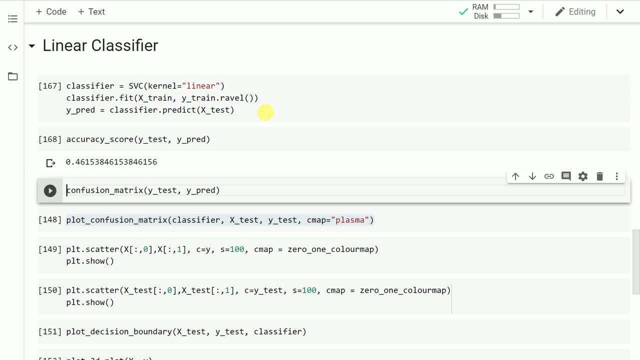 considering it's a binary classification problem And, given the capabilities that support vector machine has to offer, I expected a better accuracy score. So what exactly went wrong? before we move on to what exactly went wrong, let's also visualize the confusion matrix in order to understand how our classifier is performing. So let's run this cell as: 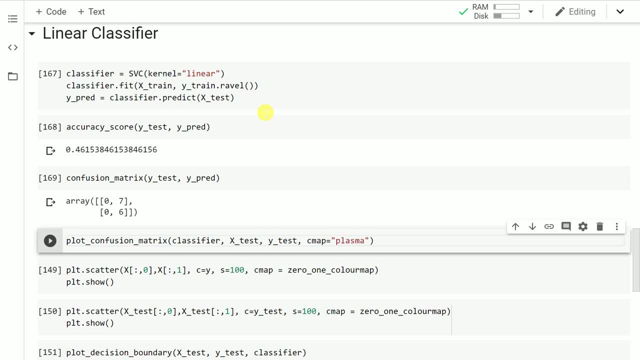 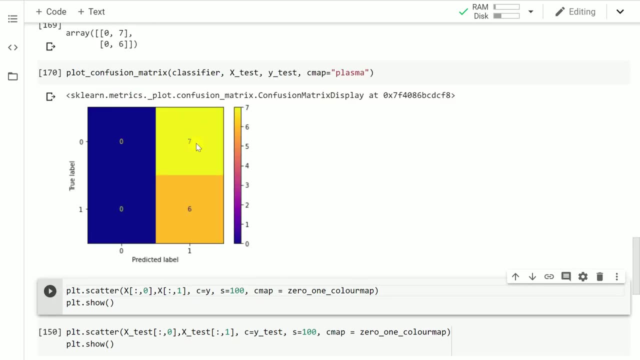 you can clearly see from my confusion matrix that some of my negative samples- that is, 0. classified as 1.. So, as you can clearly see, 7 of my samples, which were actually 0, are classified as 1, which is a clear case of false positives. My true positives are, as is so. 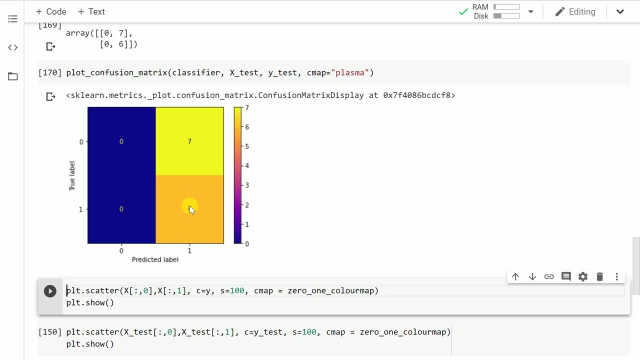 I don't have to worry about the true positive case. I don't have true negatives and false negatives in my setup, So that is where I have to now visualize a data set to understand where we've gone wrong in the whole process of building this support vector machine model. 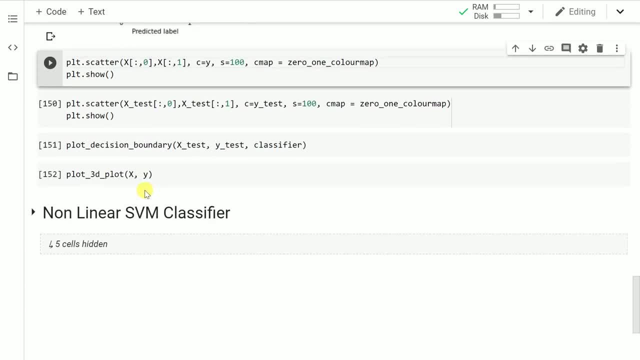 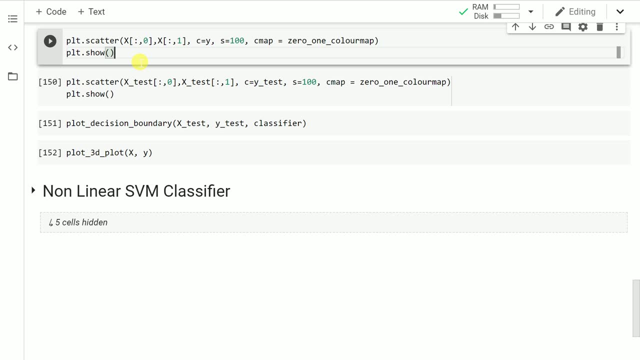 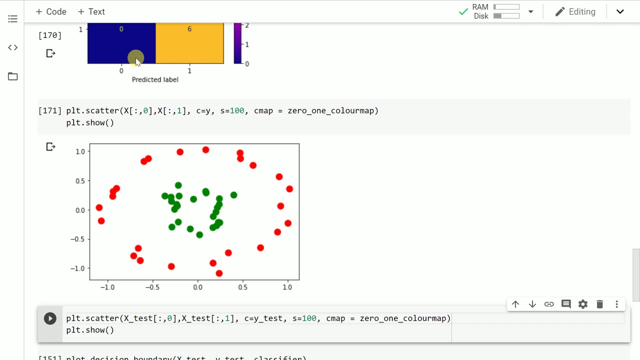 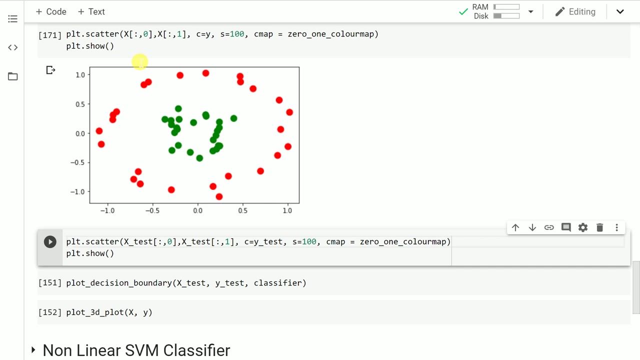 So let's move forward. Let's now try to understand where our mistake was when we created the support vector machine model. Let's now plot a scatter plot to understand how our data actually is. So, as you can clearly see, I have two features, x1 and x2, and I have a target. 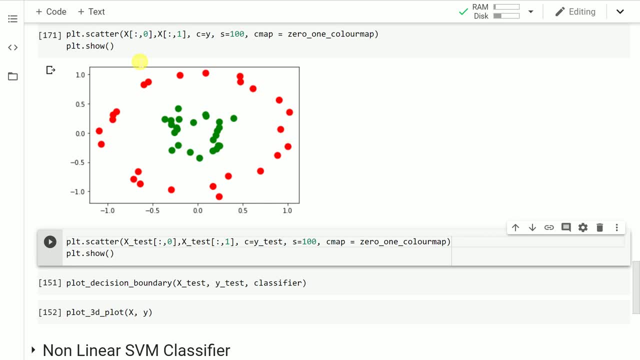 variable y. The green dots signify that these are my positive class samples, that is 1.. The red dots signify the negative class samples, which are 0.. So, if you notice carefully, I cannot draw a simple single line that would separate my class 1 values and class 0 values, which is where any linear classifier would. 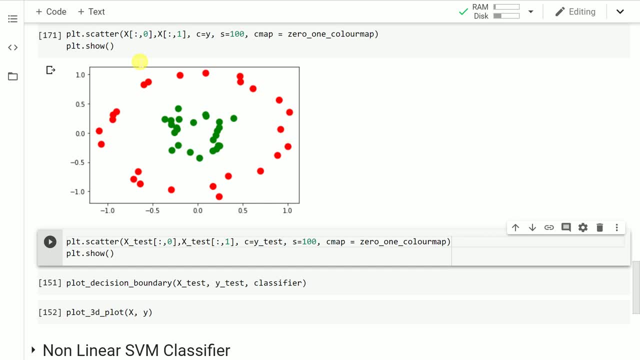 fail because my data is not linearly separable. So think of it this way: I cannot have a vertical line that can separate the two classes, Neither can I have a horizontal line that can separate the two classes. So essentially, any linear classifier with any modifications wouldn't be the best possible solution for 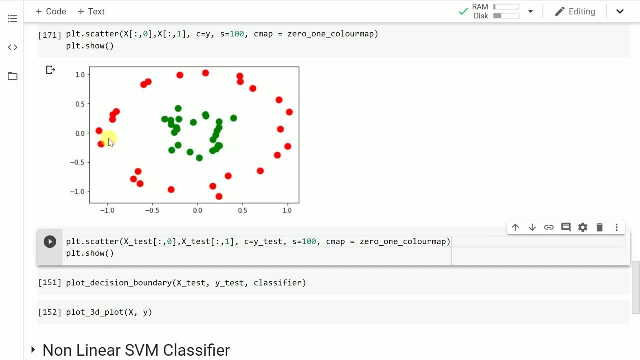 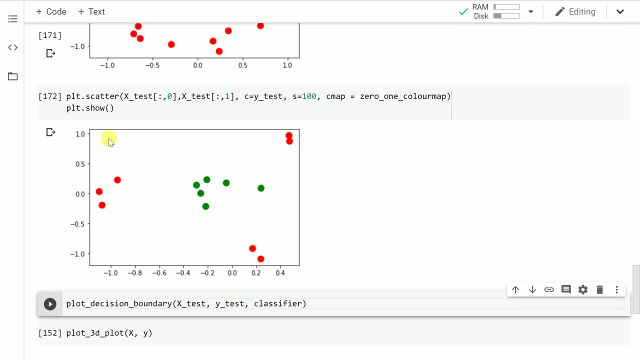 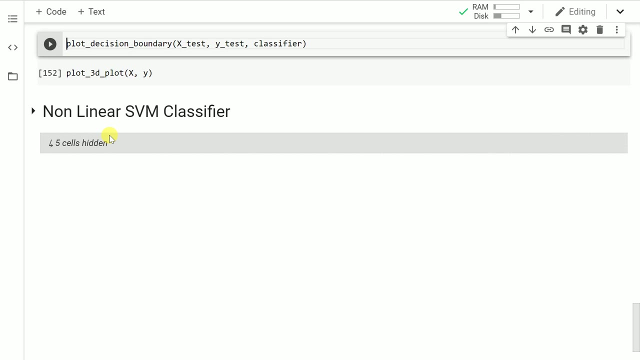 my underlying data set. If I go on to plot the X-test data as well, you will observe something similar. You can never have one single line that can separate your positive and negative class samples. Now, if you recollect, In the starting part of the video I had mentioned that I have created a function that could 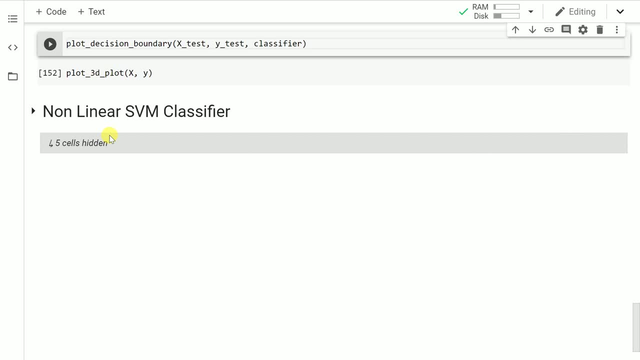 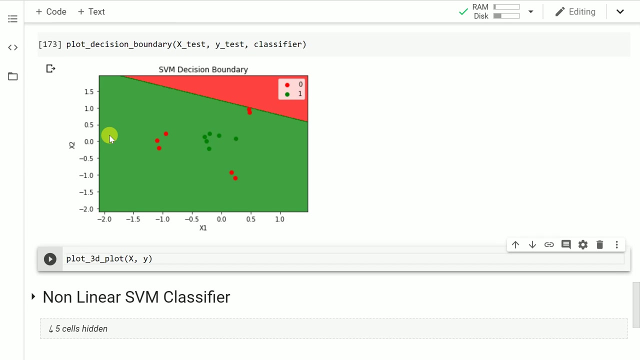 help you visualize the decision boundary of a classifier. So what I do next is I basically plot the decision boundary that I am getting using the linear SVM classifier. So let me run this cell. So, as you can clearly see, I have points such as 0s and 1s, So my 0s are listed with red. 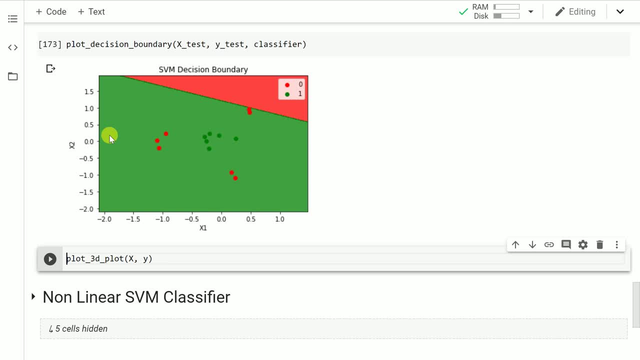 dots And my 1s are listed with green color. now my decision boundary is this line that is trying to separate the two classes into zeros and ones. so the red region is where all the points would have been classified as zeros. the green region is the region where all the points are classified as one. so essentially, 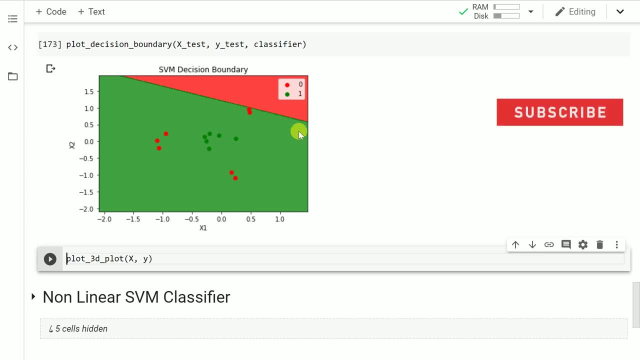 in this case, since this is my linear boundary, that is, separating the two classes, or intending to separate the two classes, what I observe is all my red points, that is, all the points which are actually zeros, are being classified as one because they lie in the green region. 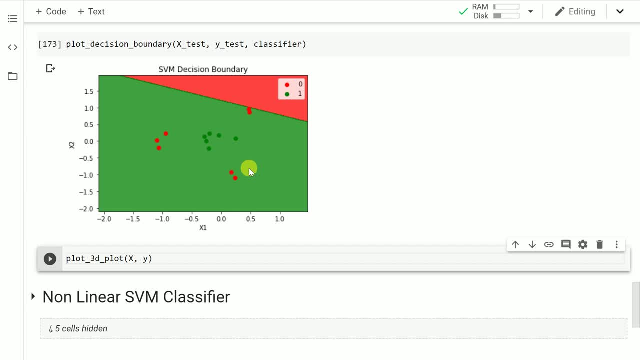 so that is why we are going terribly wrong in terms of our accuracy score, because all the points which are actually zeros are also being classified as ones. so what do we do next in order to make the SVM work really accurately? SVM has an option called as the 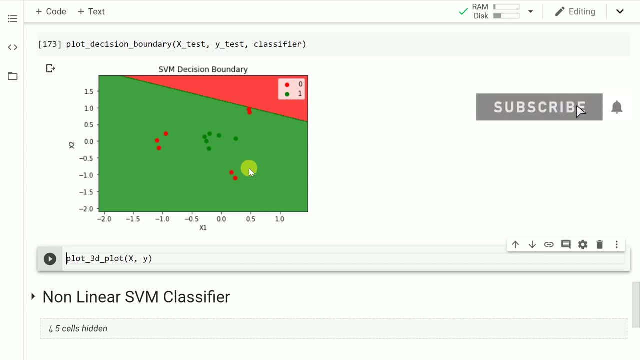 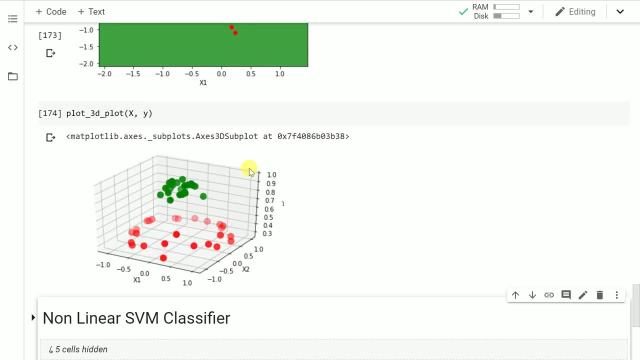 kernel trick. Now what kernel trick is? The kernel trick essentially does is: let me first kind of help you visualize the plot and then we can kind of talk more about it. So this is a simple three-dimensional plot that I have plotted. Now, once you realize that your data is not linearly separable, you specify something called. 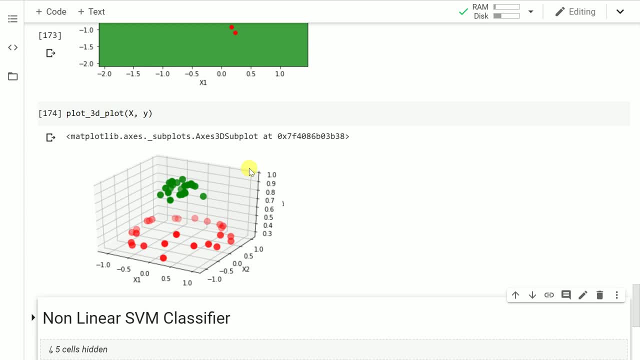 as RBF in your kernel, which is radial basis function. so essentially what it does is it takes your two-dimensional data and it projects your two-dimensional data into a three-dimensional space, such that the points which form a cluster are separated by some distance, or points which 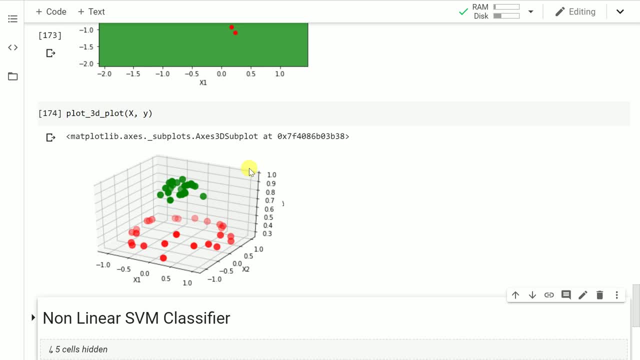 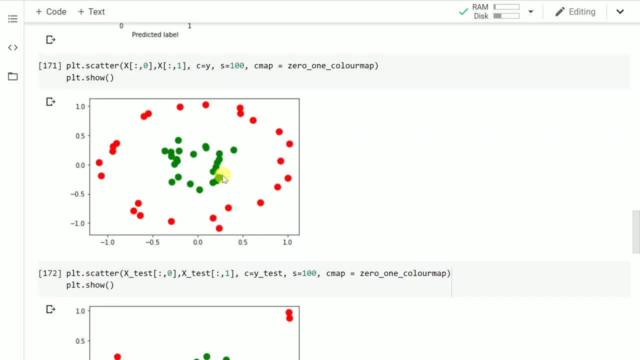 are near together would stay near in the three-dimensional or the third dimension that is added. so, for example, we had such a plot in hand, which is this scatter plot. now, essentially these were points which were of class zero, these were the points which were of class one. so, once 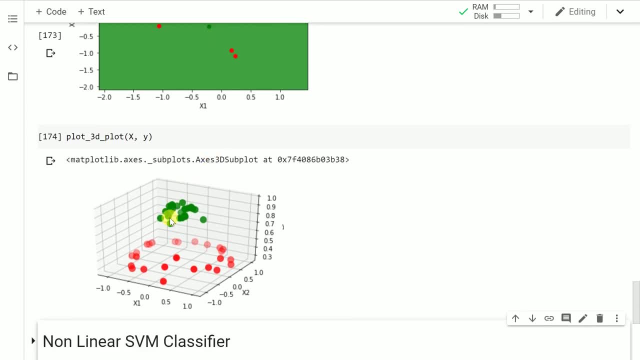 you apply RBF or radial basis function, What it does is essentially it groups the points which are similar together in terms of being collected together and expands it to a new dimension with a different distance. so these points are concentrated, say nearby together, so they occupy a specific Y location. 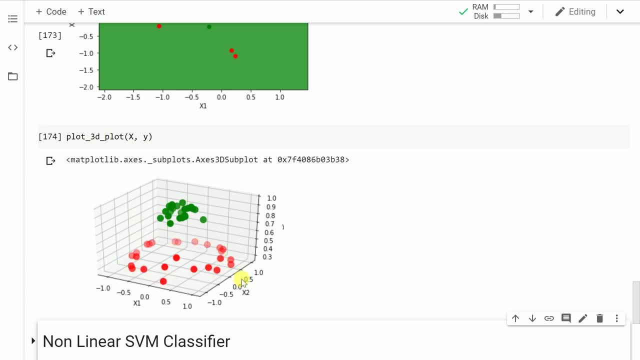 if you consider this as a 3D plot, and these red points are scattered together, so now they remain at a particular Y location itself. so now it's able to kind of create a three-dimensional space which is linearly separable in a higher dimension as compared to something which 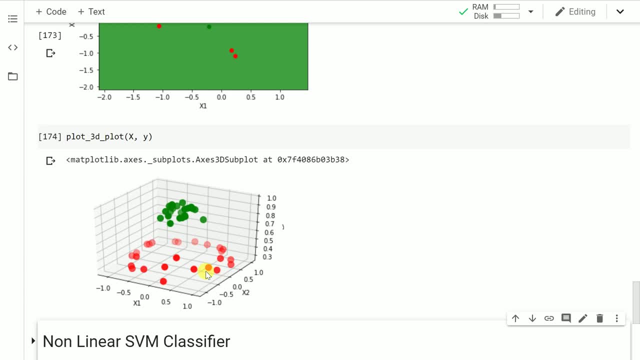 was non-linearly separable in a lower dimension. so it's added a dimension, it's grouped points which are, say, close together in a different space and thus creating a higher dimensional space which is linearly separable. so that is the advantage that you get once you use. 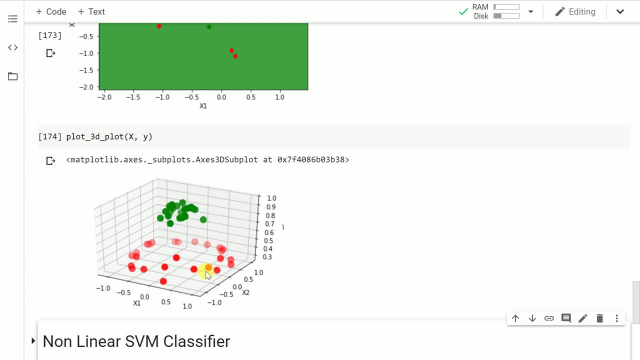 RBF. so this was a small projection that I had in mind in terms of explaining you how say the kernel trick works. so there are different kernels which are available. one of them is RBF, wherein it kind of tries to figure out which are the closest points together and 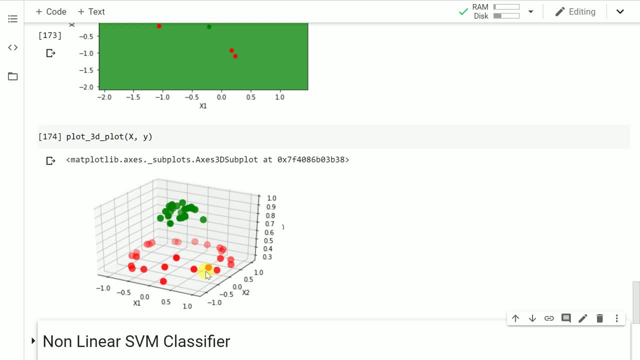 it then translates those points into a particular direction, so that you can kind of have linearly separable data in hand. now that we've looked at how radial basis function works or the RBF kernel trick works, let's now go on to explain this using actual code and see if 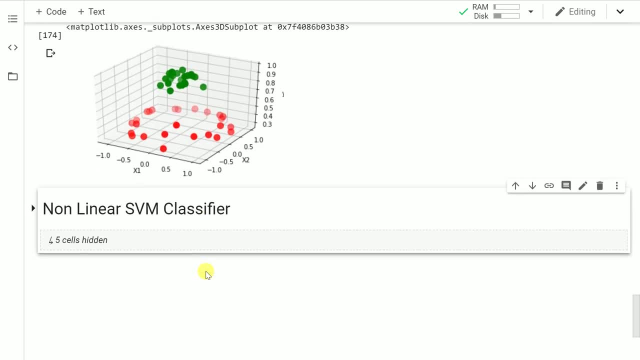 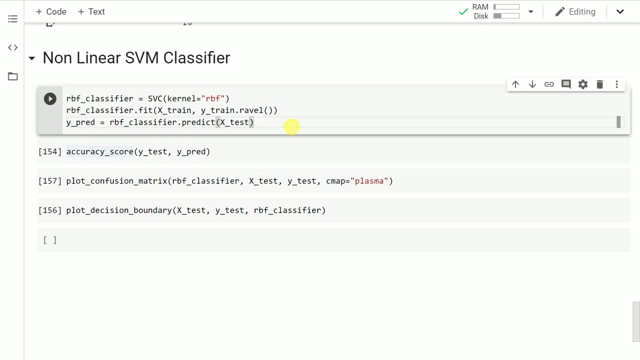 our accuracy is correct, Improves or not, so let's move forward. I follow the same steps that I followed while creating the linear SVM classifier, the only change being now I change the kernel from being linear to RBF, which is the radial basis function. I fit my training data, that is, X train, and. 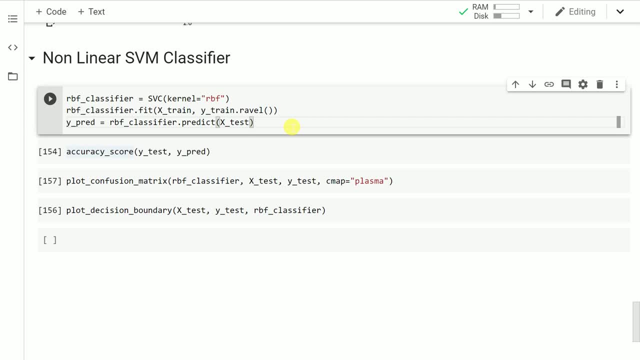 Y train. I catch hold of the predictions by the classifiers predict function by passing in the X test values and I save the values into a variable called as Y train and I save the values into a variable called as Y train and I save the values into a variable called. 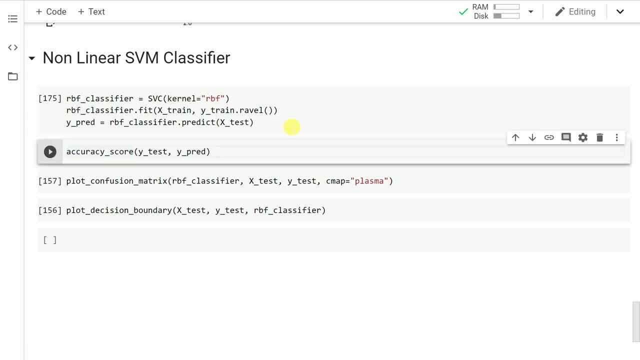 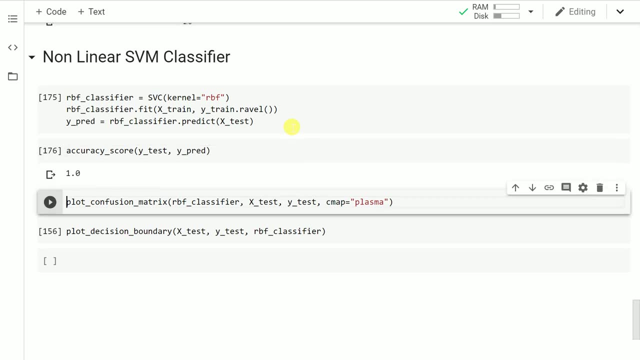 as Y train and I save the values into a variable called as Y underscore pred. so let me run this cell now. the cell has executed, so let's go on to calculate the accuracy score. now, since this was like a small data set that I was playing around with, I observe a testing. 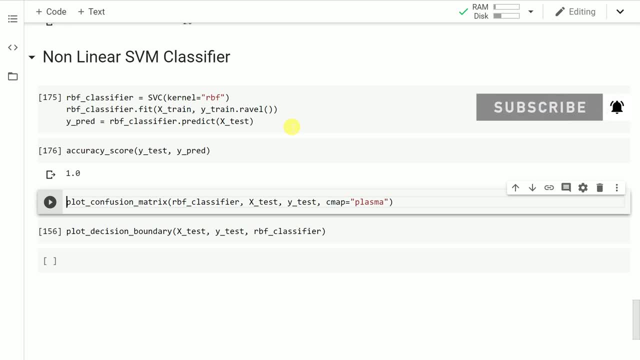 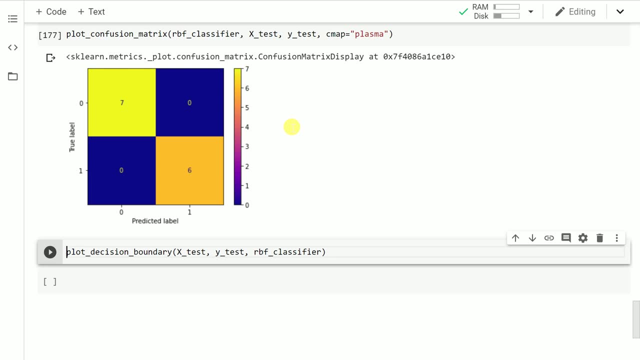 accuracy of 100%. let me now plot the confusion matrix. as you can clearly see, there are seven true negatives. that means all the samples which were zeros are now correctly classified as zeros and all the samples which were once are now correctly classified as ones which we had as six samples which are now correctly classified as once. so I have two positives. 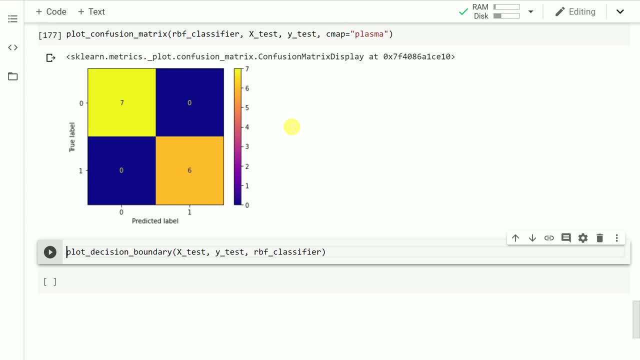 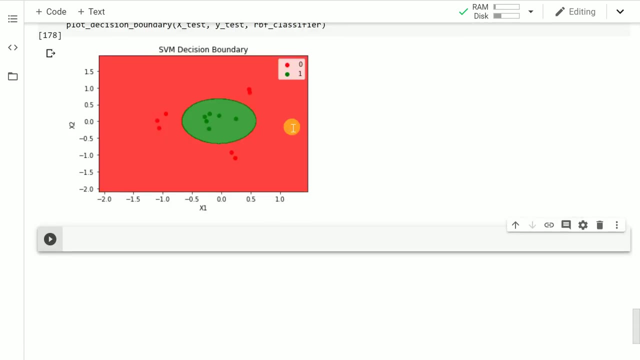 I have two negatives. all of them add up to 13. I have total 13 samples in my testing data set and I don't observe any false negative and false positive. now let's go forward and also plot the decision boundary. Now, if I plot the decision boundary in two dimensional space, this is what I observe as 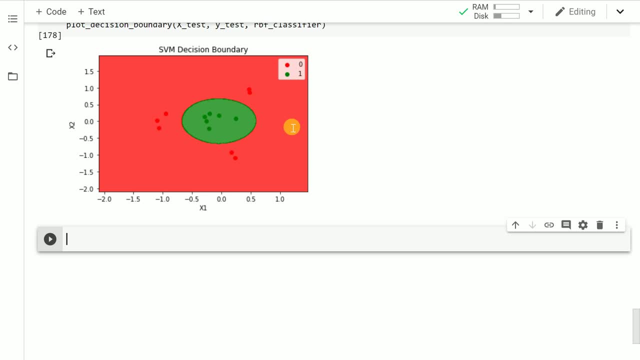 you can clearly see, this is more like a circular boundary that's being bounded based on the data that I have provided. so this is how the kernel trick can kind of give you a nonlinear boundary in two dimensional space, but think of this nonlinear boundary as a linear plane. 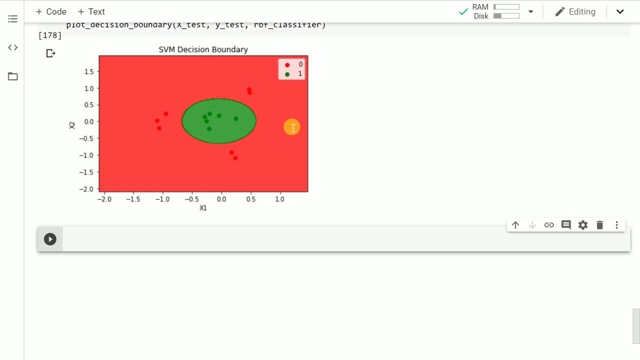 in the three dimensional space. So this was my attempt at explaining how support vector machine gives you that power of creating a very accurate decision boundary. I hope you enjoyed the video. if you do have any questions with what we covered in this video, then feel free to ask in the comment section below and I'll do my best to answer. 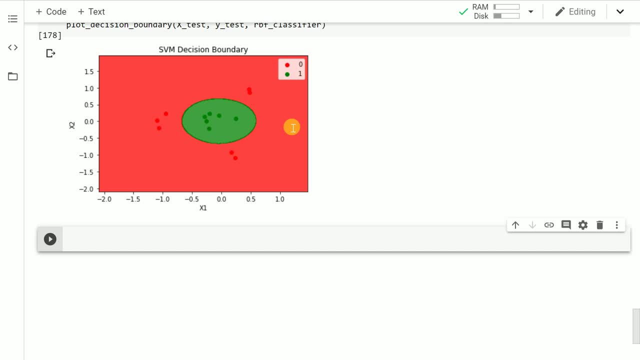 those. if you enjoy these tutorials and would like to support them, then the easiest ways to simply like the video and give it a thumbs up, and also it's a huge help to share these videos with anyone whom you think would find them useful. Please consider clicking the subscribe button to be notified for future videos and thank. you so very much for watching the video.